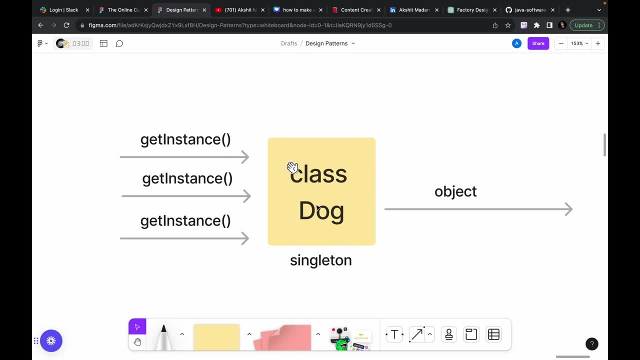 right, That means only one object. So for, let's say, if this class dog is now a singleton class, I can only create a global object, single object or I can say single global object of this singleton class dog. And the process of creating objects of the singleton class is quite different. 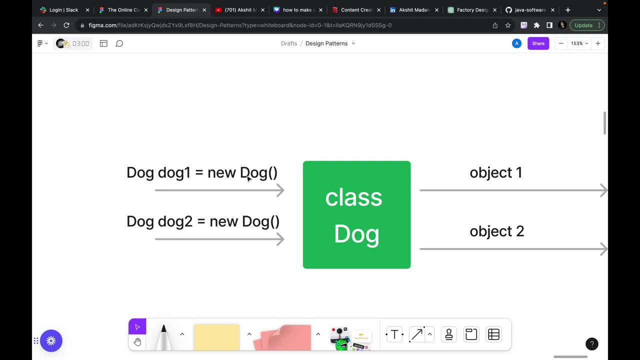 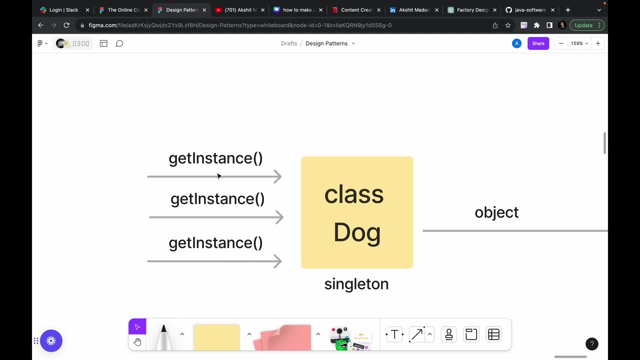 You cannot use this syntax class name. object name is new class name. You have to define a get instance method inside this, inside this class. This method is going to be static. So I can say that this get instance method is going to be static. 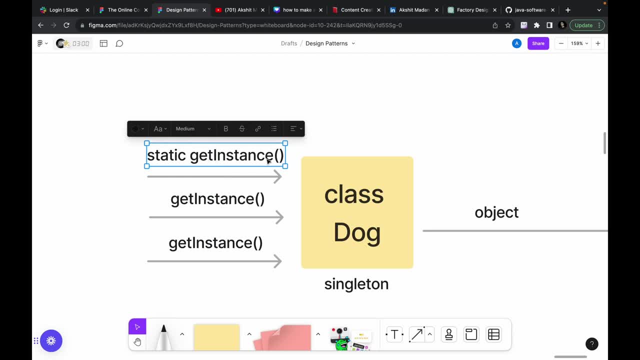 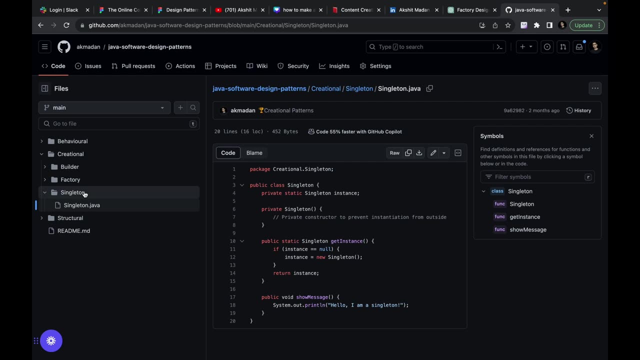 So I can say that if any method is static for a class, you can access this method from anywhere without creating the instance of this class Right Now. let's see the code example using Java. Now I've come to my code files. So you can see that I have a package called singleton which is inside a 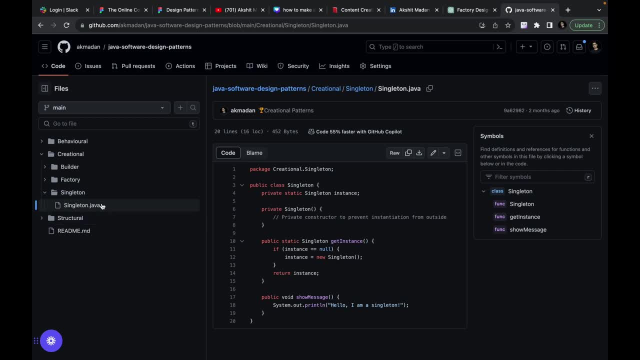 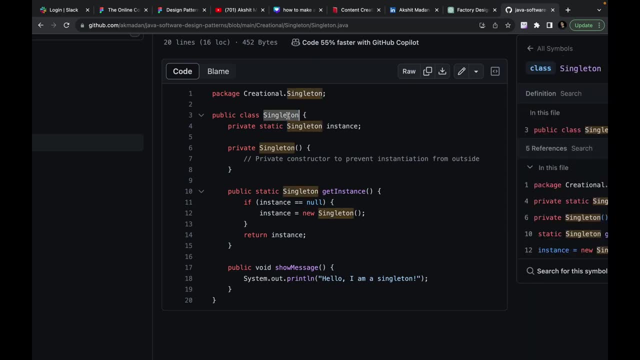 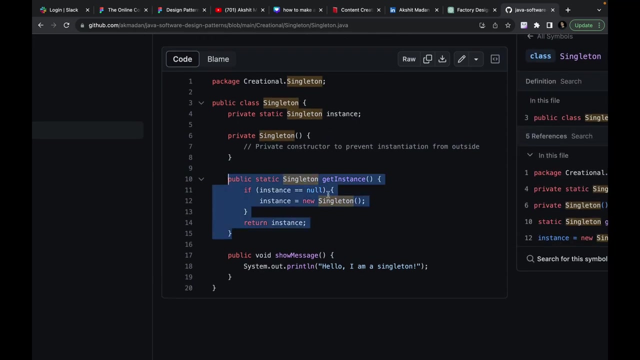 package creational. right Now, inside the singleton package, I'm having singleton dot Java. Now we are going to focus on this class. It is a simple class, public class, singleton. Now this class can be any class name. It can be cat, dog or anything. right Now, focus first of all over here. So first of all, 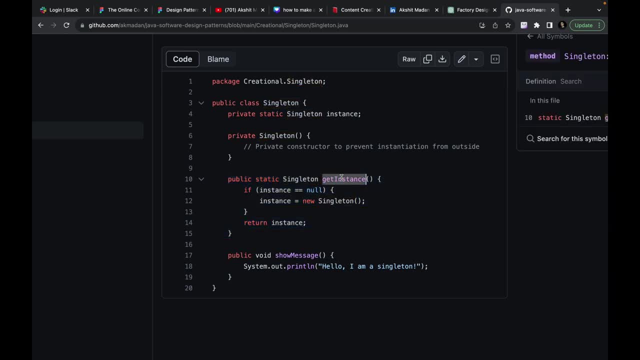 this singleton class is having a function get instance, right, And this is a static function. Now, because we have made this get instance a static function, that means you can access this function from anywhere using this class name: singleton dot. get instance As soon as you're. 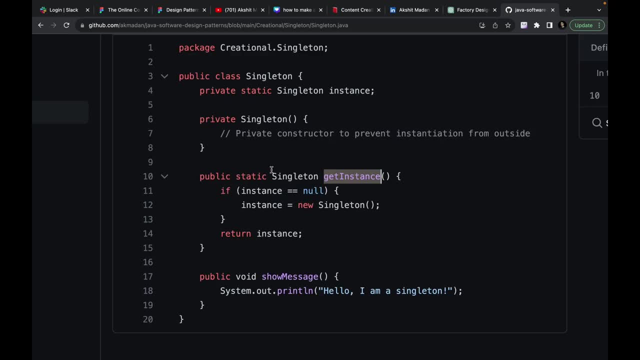 going to do what this function is doing. If my instance- this is my instance- right, This is a variable which is going to store my instance. If it is null, that means I have not yet created any instance of this class. If yes, I'm going to create an instance- singleton- and I'm going to update this. 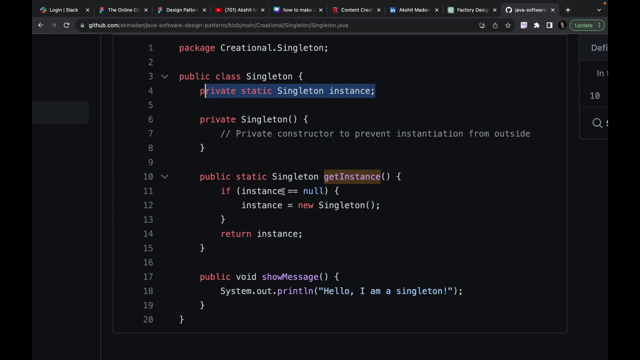 instance variable value. But if this instance value is not null, that means I've already created one instance of this class. then I'm not going to create any another singleton object. I'm just going to return this instance which was previously created. 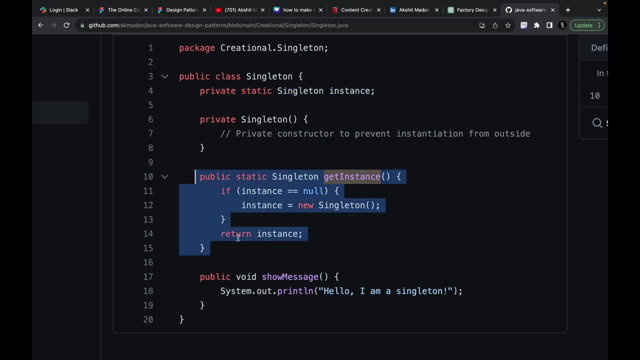 Right, That's it. That's it. This clearly shows that you cannot create multiple instances of this class. You can only create a single instance, store it in a variable and return whenever, the whenever someone wants to create an object of this class. Now, this private function.